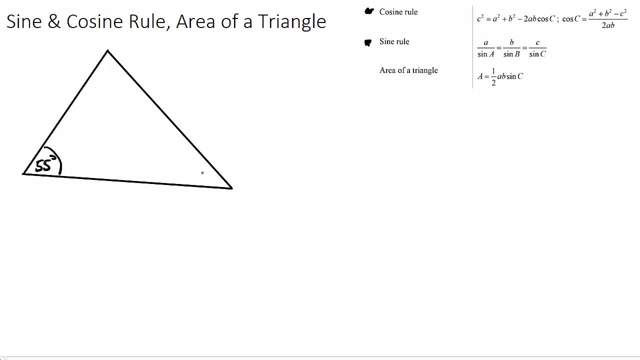 say 55 degrees, and this one here was- I'll use- 48 degrees, and we knew this side length here was 12 centimeters and we want to find this side length here X. Okay, we are given enough information because we are given two. we are given. 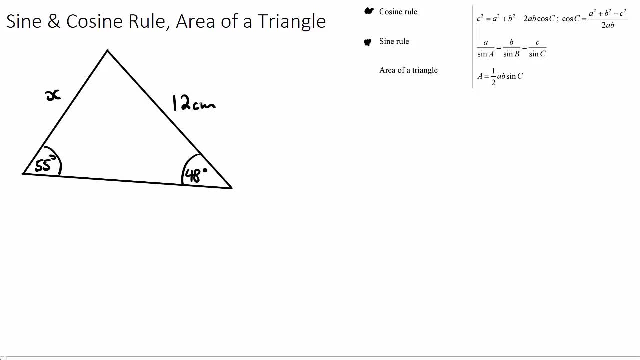 two angles and we know one side length and we want to find the other side length. If we have two angles and a side length and we want to find another side length, we need to use the sine rule, because the sine rule says: if in a 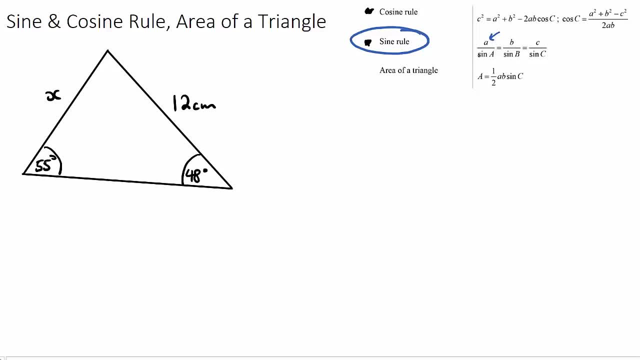 triangle. you take any side length and divide it by sine of its opposite side length. so the A and the capital A are linked. the lowercase a means a side length and the capital A means the opposite angle. this is equal to another side length over the. 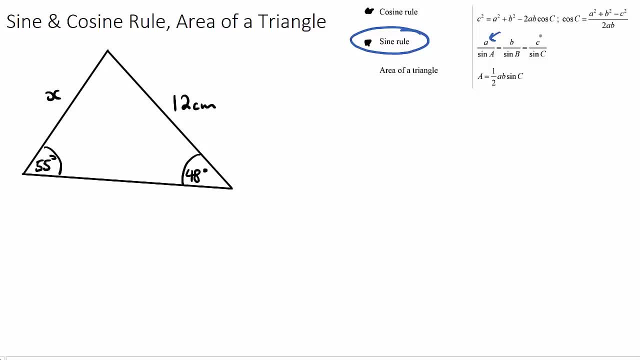 sine of its opposite angle, And they have this equal C as well. it just demonstrates that if we take any side length and divide it by sine of its opposite, you can make it equal to another side length. So you only need to use two of these when you use the sine rule. So I'm going to say that sine or A. 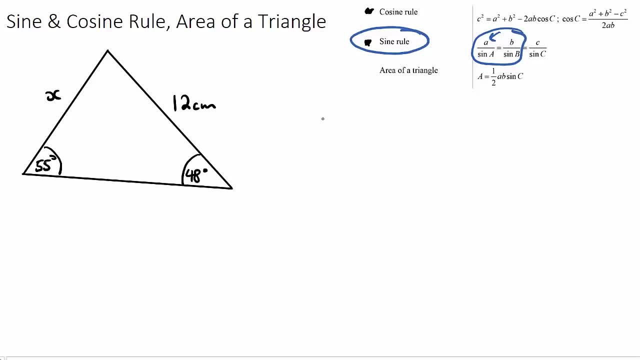 A, I'm going to use 12, so 12 over sine of its opposite, which will be 55 degrees. this will be equal to another side length, which will be X over sine of its opposite side length, which would be 48 degrees. And I have an equation here where 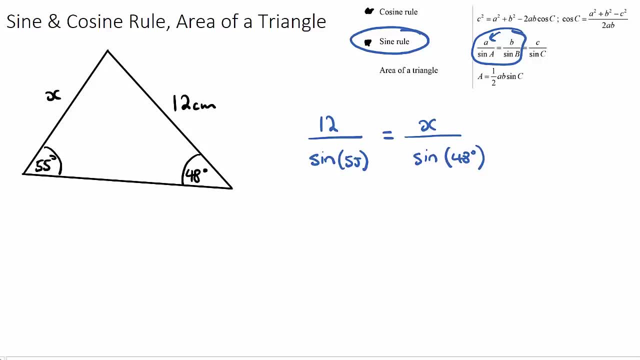 X is my only variable. I can solve for X, which is my side length, And I can do that just by multiplying the sine 48 up on the other side. So 12 multiplied by sine of 48 over sine of 55, this will equal X. And if we can do this on our 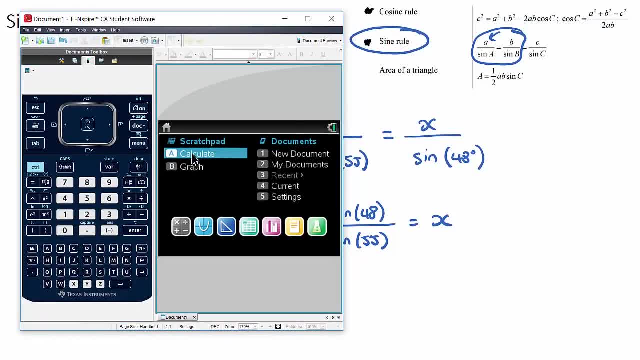 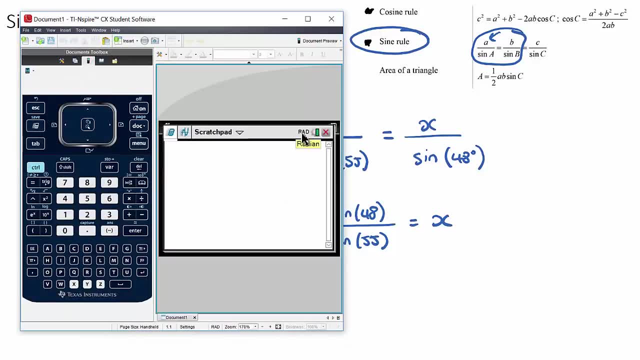 calculator, we can solve our answer, So I'll just quickly do it Now. we need to be in degrees, because the angles that we are using here are in degrees, so make sure we are in degrees mode. So I'm in radians here, so I'll just change to degrees. 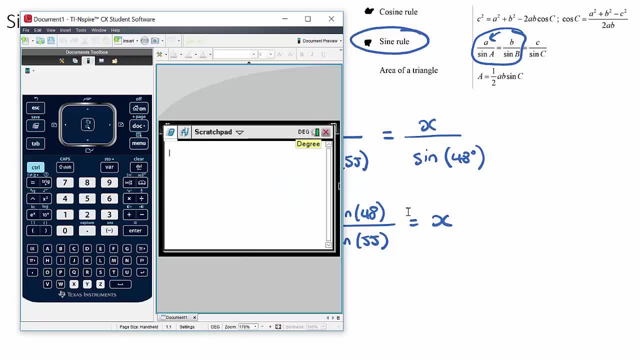 Okay, now we have degrees. So X was- let's set up our fraction- 12 times sine of 48 over sine of 55.. Okay, so X is 10.9. for three significant figures, X would be 10.9. 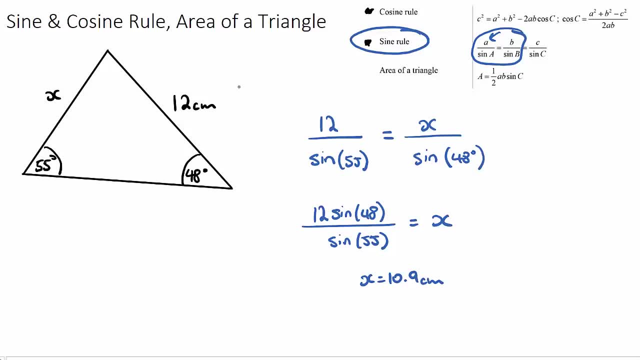 centimeters. Okay, so we use the sine rule. if we have two angles, one side length and we want to find another side length, I'll change this. now. What if? okay, I'll give this one now a different one. So this was given. Let's say, this was 10 centimeters. 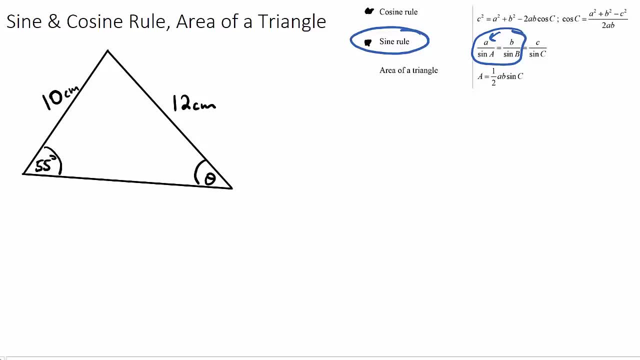 and we want to find theta. So now we want to find an angle. Well, still, we have two side lengths and one angle and we want to find another angle. We will once again use the sine rule, because the sine rule has two of both and we can solve for one of them. 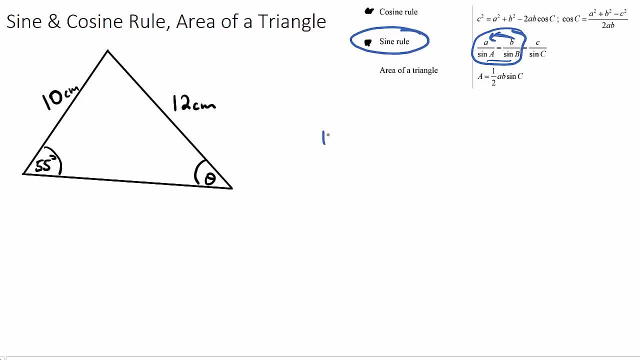 So what we would do there is we can actually say 12 over sine of 55 will be equal to 10 over sine of theta, and we want to solve for theta. Now, what you'll notice here is it might be a little bit tricky to solve for theta, as 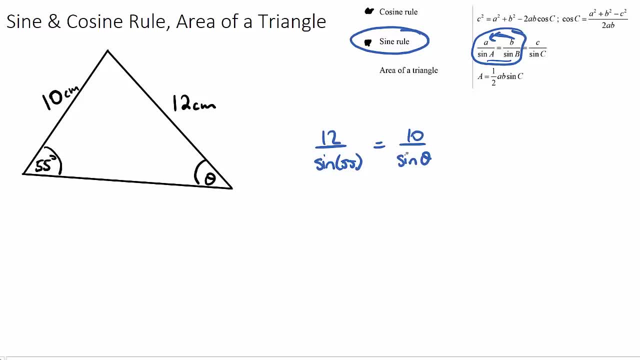 it's currently on the denominator, but what we can do is we can actually flip both of these fractions. sine of 55 over 12 is equal to sine of theta over 10. And that makes it easier because we can simply multiply the 10 up 10 times. sine of 55 over 12 is equal to. 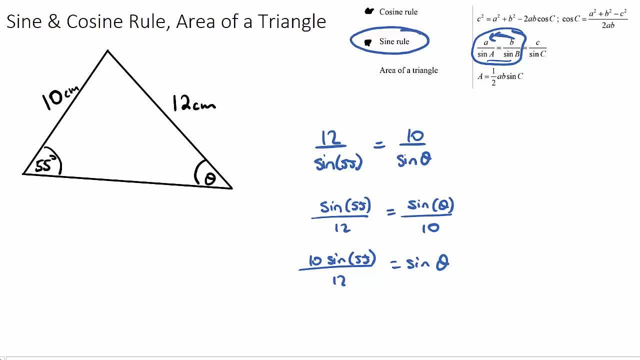 sine theta. Now what I did there? by flipping both sides. you can do that as long as you do it to both sides of an equation, And in some textbooks you might see this sine rule actually flipped. It might have all of the sine a and sine b. 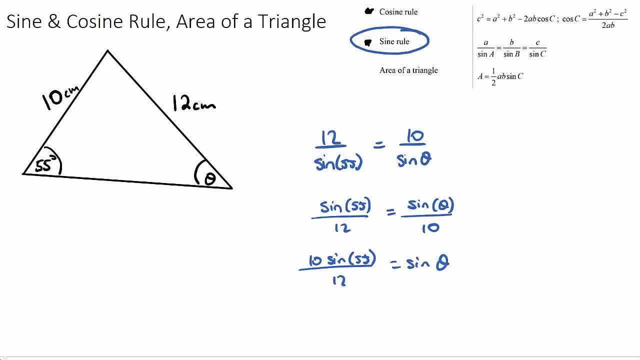 and sine c on top and the a b, c on bottom, which is perfectly fine, So you can use either of them Now to solve for theta. here we need to go sine to the negative 1 and we need to put all of this in here So we can do that in our 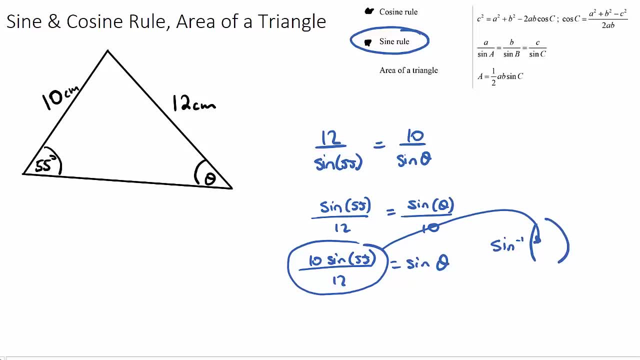 calculator and we would solve for theta. Okay, so that's using the sine rule. I will show you the cos rule, And the cos rule is useful if we have three side lengths. Let's have a look at the cos rule. The cos rule here is useful if you have three side lengths, for example c, a and b, and 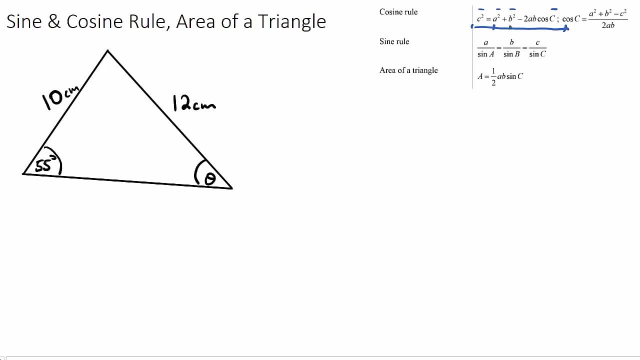 only one angle. So if you'd have two of them given and the angle is given and you want to find a third side length, we would use this first cosine rule equation up here An example of that. Let's put in our value here. Let's say we want to find x And notice in this: 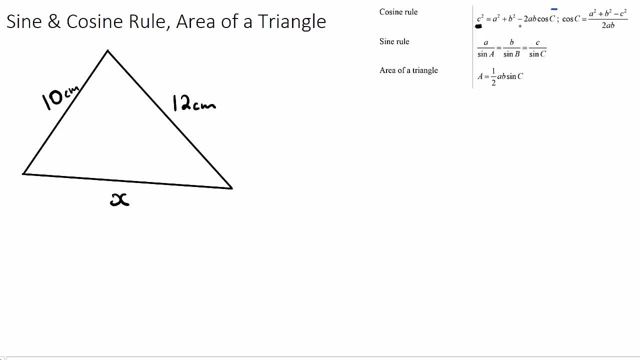 equation, the one that we want to find, which would be c. we need the opposite angle, So this one needs to be given. This might be, let's say, 60 degrees, And if we we have two side lengths and an angle and we want to find a third side length, 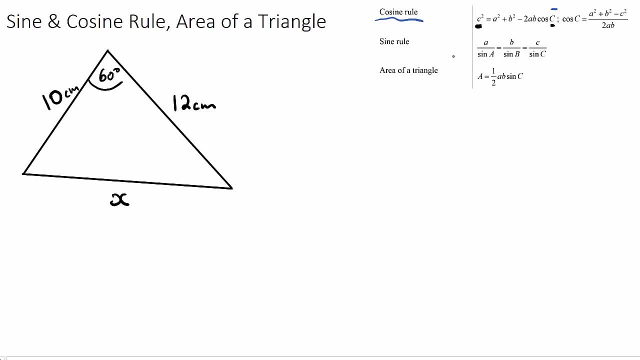 that is when we use the cosine rule. The sine rule wouldn't help us here to find another side length. So we would say x squared is equal to the other two lengths squared. So 10 squared plus 12 squared minus 2 times those two side lengths multiplied by cos. 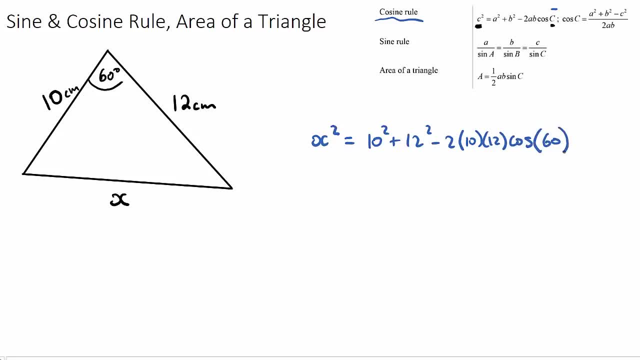 and we have the opposite angle, And then you would simply just type this into your calculator and you would get some number for x squared, and then we just take the square root of whatever. that is Okay. so the cos rule is useful if there are three side lengths involved. You might. 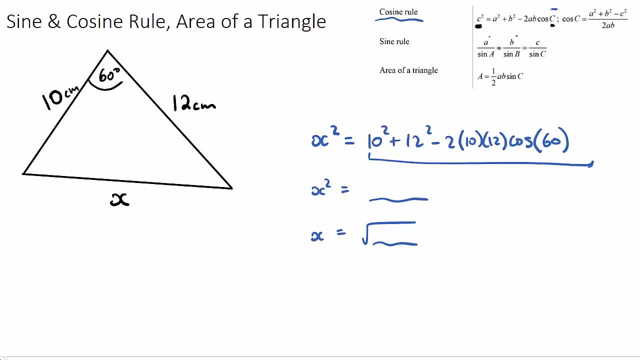 not have all three, but the sine rule is only when you have two and two, And the other cosine rule is actually the same. This cosine rule here is the same as this one here. They've just been rearranged, And this one- the second one is useful if you are given three side. 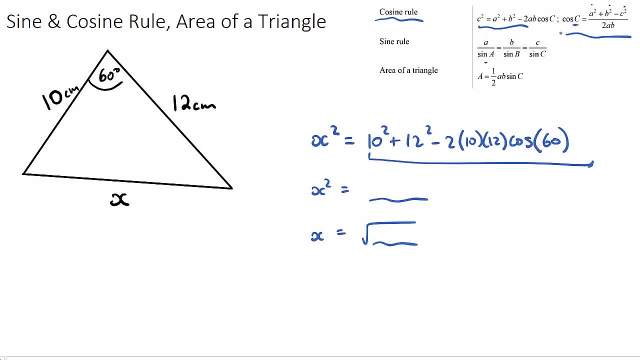 lengths and you want to find some angle. You can use the rearranged cosine rule to find any angle. And those three side lengths, Okay, and finally the area of a triangle. The area of a triangle. we use this last formula down here.